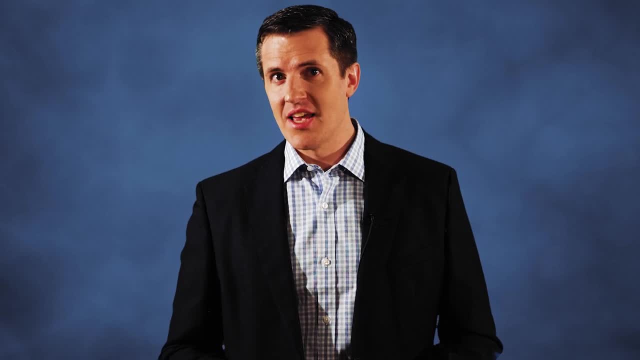 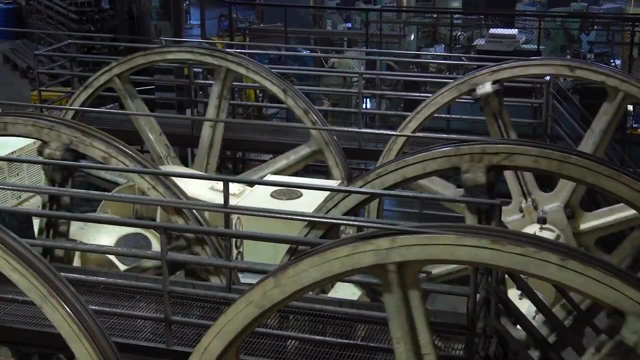 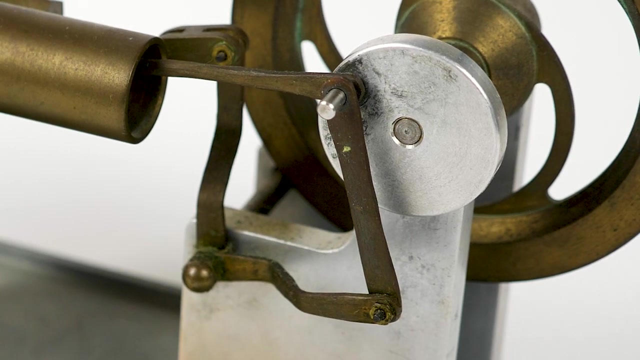 building blocks that constitute mechanical systems, such as cleverly shaped rigid bodies, gears, pulleys, belts and sprockets, to name just a few. I'll teach you how these building blocks can be joined together to create a system that can be built on its own. 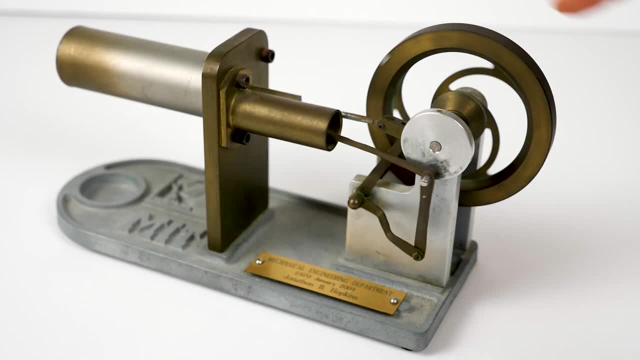 The first thing we need to do is to flash these blocks. The first thing we need to do is to flash these blocks using traditional rigid joints such as revolute and prism joints that guide their bodies in complex ways to achieve extraordinary tasks. Specifically, you'll 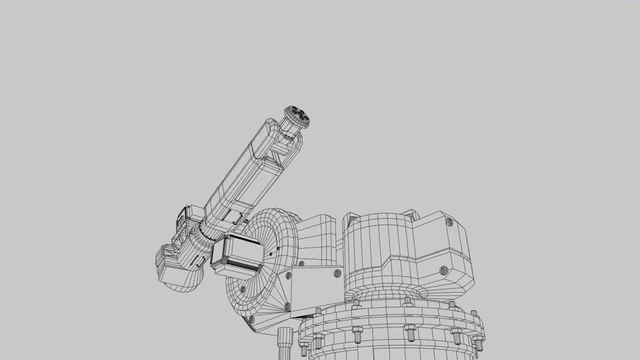 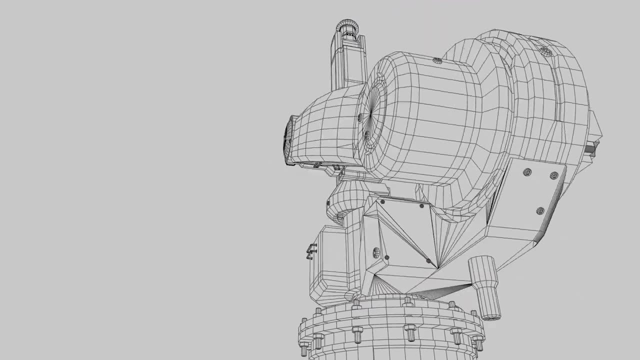 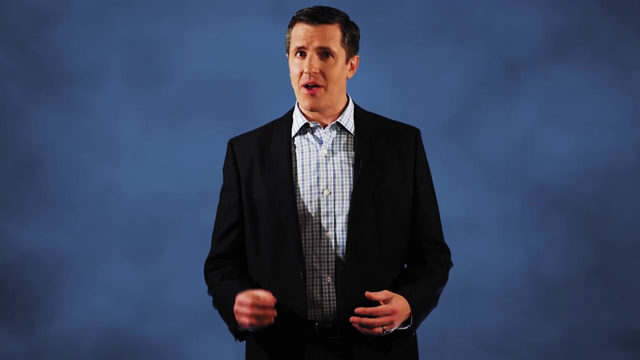 learn how to analyze the position, speed and acceleration of every point on any body within a moving mechanism, as well as calculate the forces and moments that the moving mechanism experiences. Now you might be wondering why I would teach a class about traditional rigid mechanisms when my area of expertise is compliant. 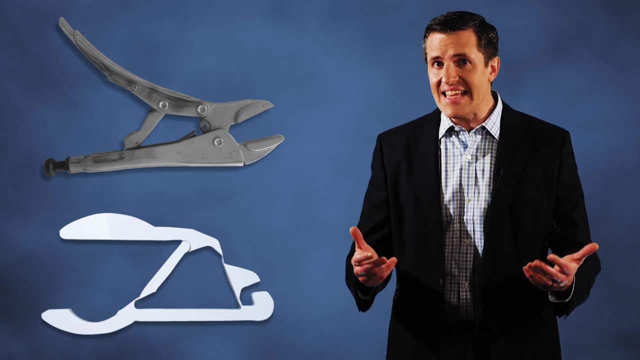 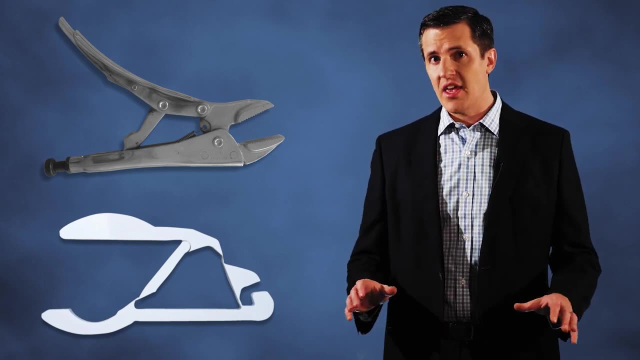 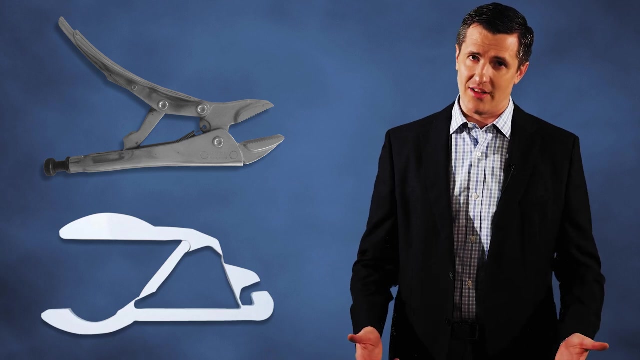 mechanisms. Well, the reason is that it's easier to understand the principles of analysis in the context of rigid mechanisms first, But trust me, many of these same principles can be applied to determine the kinematics and kinetics of compliant mechanisms as well. If I have you excited to take this course, I'm glad. 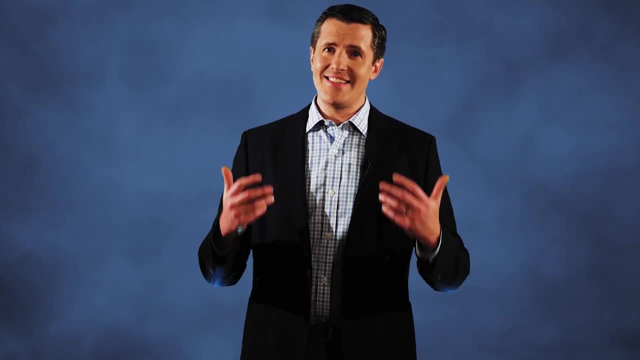 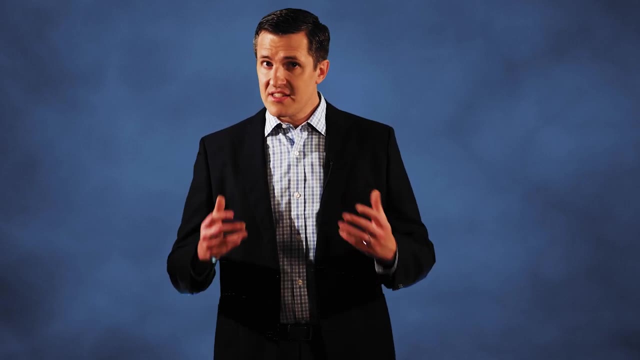 but don't be deceived: This course is a free course and it's free to take. This course is not as engaging or entertaining as my Compliant Mechanism Design Professional Video Series, Similar to my Compliant Mechanism's Lecture Series. this 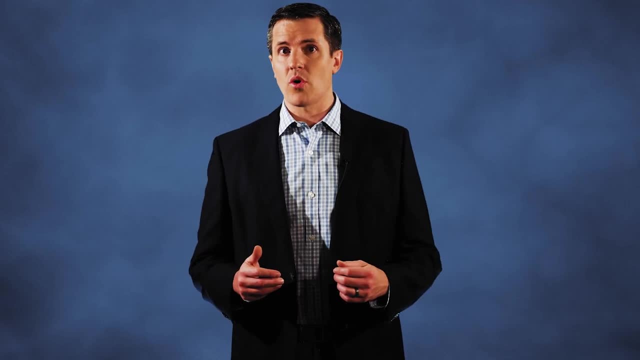 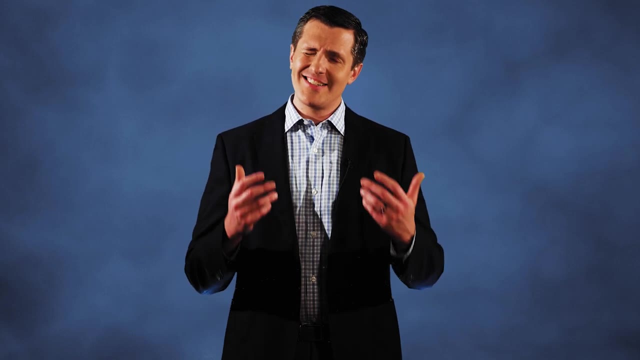 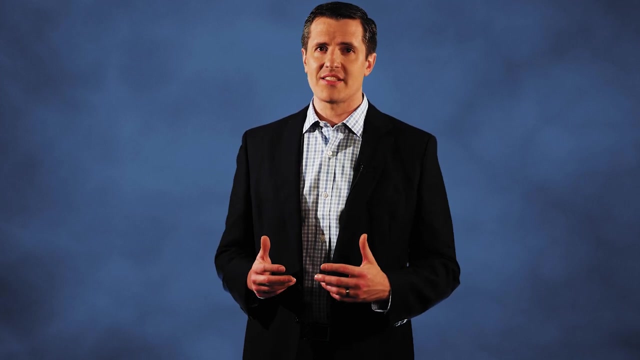 course consists of raw, unedited recordings of the actual lectures that I use to teach my undergraduate students at UCLA, so these videos are not suited for everyone. They consist almost entirely of college-level mathematics and thus aren't generally accessible to everyone. This course is a free course and it's free to take.